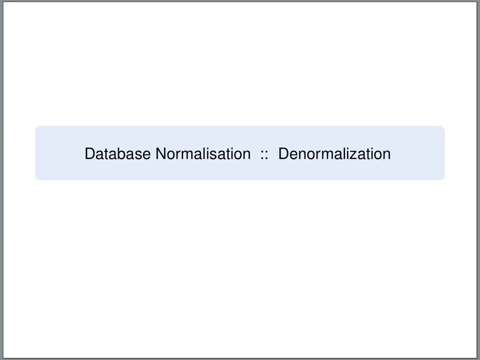 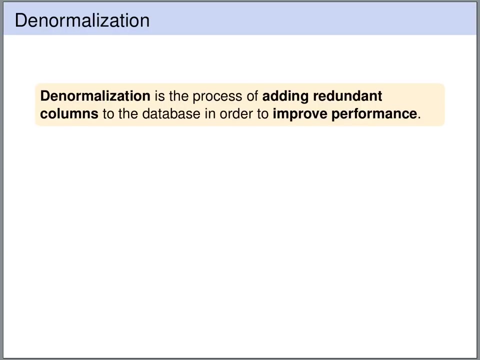 The goal of database normalization is to avoid redundant storage. Sometimes, for the purpose of performance, it is necessary to violate the normal forms and to intentionally introduce redundant storage of information, And this process is called denormalization. Denormalization is the process of adding redundant columns to the database in order to improve. 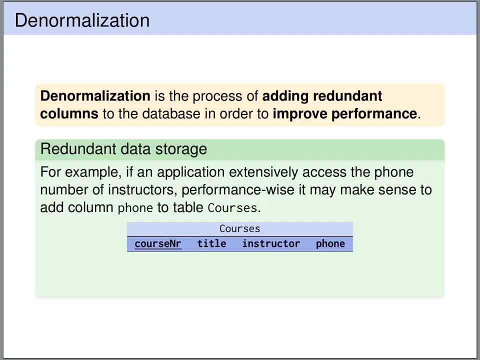 performance. Let's have a look at the example that we've seen before. We have split the courses table and we've removed the phone number from the courses table. We've introduced a separate table with the instructors and the phone number. If we have an application that makes heavy use of the phone number for particular courses, 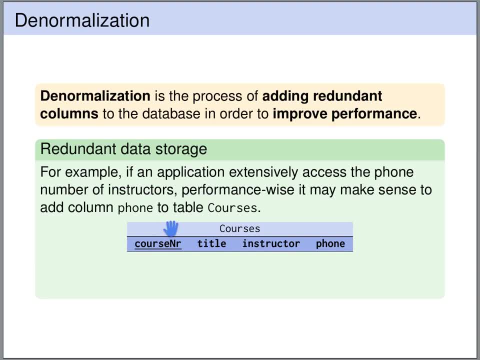 then this makes actually sense to add the phone number back into this table if we really cannot afford the performance overhead of the necessary join operations. So if this performance overhead of the join operations is too much because we're using the phone number too often, then we have to add the phone number back into this table. 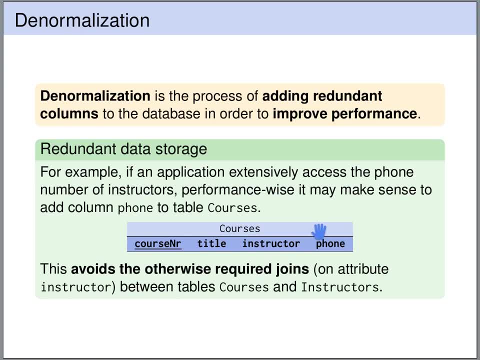 To add the phone number back into the table. we've removed this table link with the site user information So we can add the phone number back to this table. So we have redundant storage of information because we still have our separate table with the instructors and the phone number. 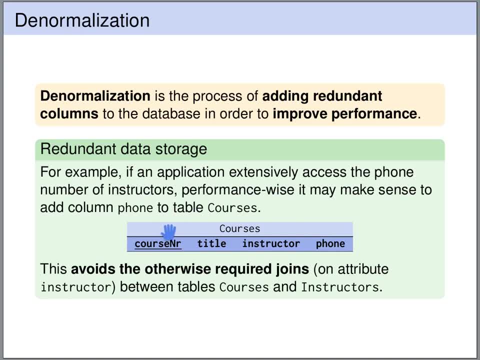 But now, if you want to look up the phone number for a particular course, we no longer need a join operation. We can directly retrieve this phone number from the courses table. We can also save the number of courses data as function. And that's it for this example. 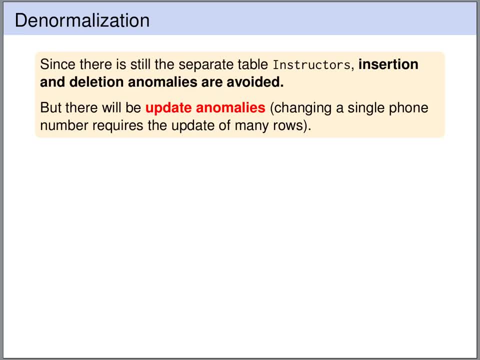 Since we still have the separate instructors table with the Names and the phone numbers for each particular course, I can add the information for each course token, And that means one of the functions in this application is only valid, one extra. I am showing you the names and the phone. 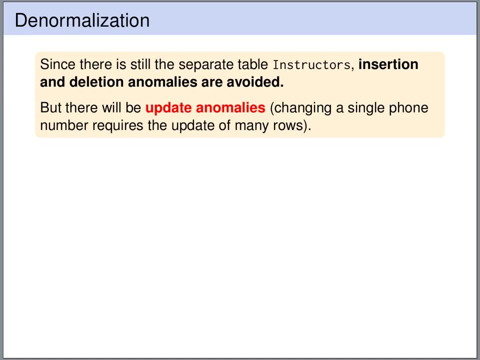 numbers of each particular course By using our turtles and put their names, for example the number of the instructors, we avoid the insertion and the deletion anomalies. We can still insert the phone number of instructors even if the instructor does not give a course. 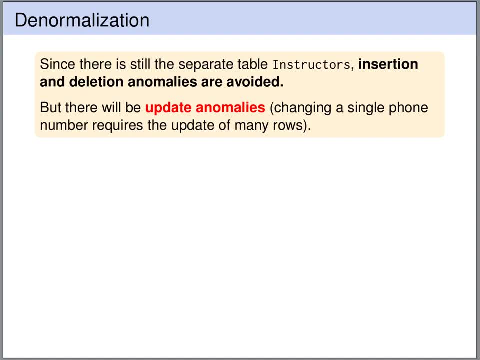 And even if the last course of an instructor is deleted, the phone number is still in the instructors table. However, we will have update anomalies. So if we want to change the phone number of an instructor, then we have to now change it in multiple positions in the instructors table and multiple times in the courses table. 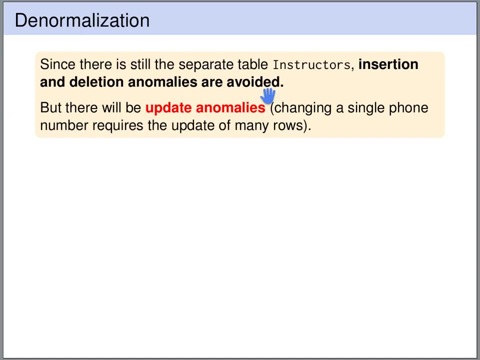 for each occurrence of the instructor in the courses table. So we have slightly faster queries to retrieve the phone number for a particular course. However, we pay for this performance improvement by a more complicated application logic. The applications have to update the phone number in multiple places. 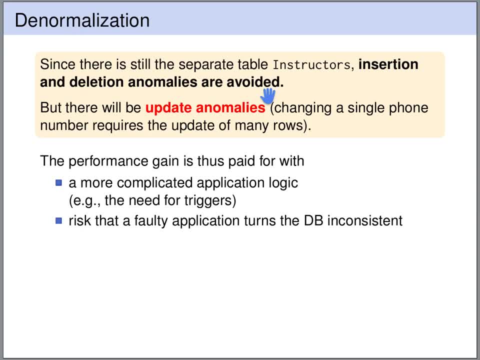 So the updates become slower because now there is an overhead of having to update multiple phone numbers And we risk that if the application that accesses the database is faulty, then this application can turn the database state inconsistent. So if you have an application that only updates the phone number in the instructors table, 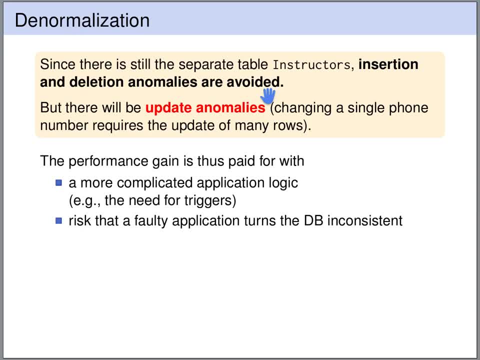 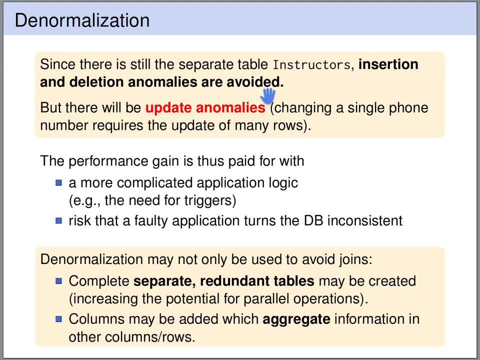 and not in the courses table. then you suddenly have an inconsistent database state, So you may want to change the function data Stricse, the application, to a new one. You can change the function data to not one, And the data state remains the same. 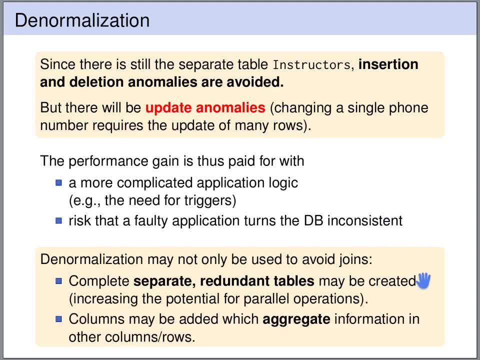 The first thing you should make sure is that the application parameters are correct. You can change the function data to be right and correct. If not, you may have to change the description to be correct. So if you want to change the function data, you should change the name to your own and 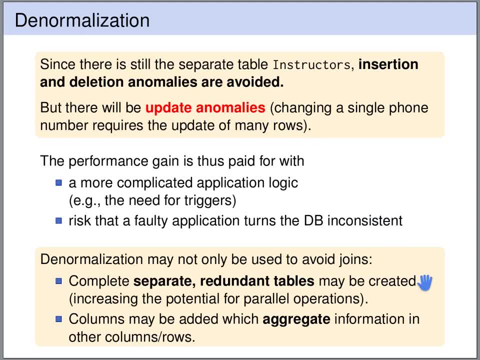 the form which you use to change the function data. Then you have to update the function data to a new one. This service can be done in multiple different ways, For instance by adding a special function in the applications. You can add a function that is address. 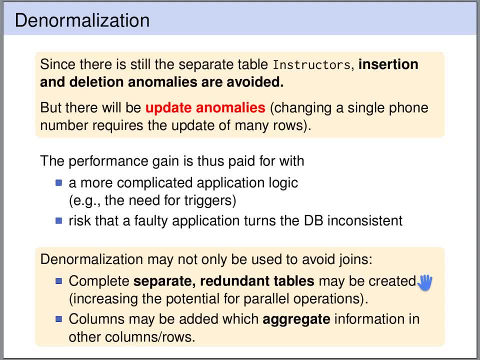 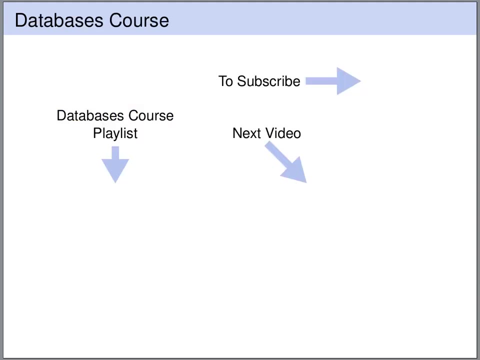 For instance, the information大的 date. So we can think of different uses of denormalization in order to make queries faster, or to simplify applications, or to increase the potential of parallel operations. Thank you.